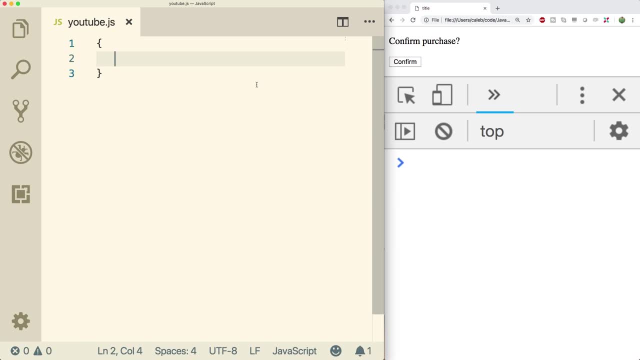 too crazy about numbers. There's just some things you need to know to understand how they work in JavaScript. but they work basically like expected. So, for example, if we have a number, it looks like that. You've probably seen that a thousand times. but one thing you need to know: 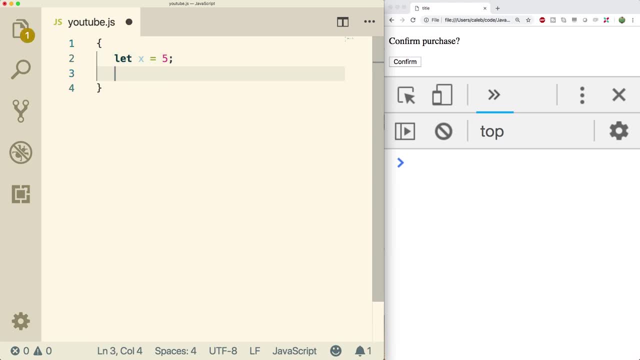 is that you can also store decimal values. So for example, we can say X is 5.5.. Internally, numbers are 64-bit floating point numbers. So this is known as a double precision floating point number and is in contrast to what's known as a float, which is just 32-bit. So 64-bit gives. 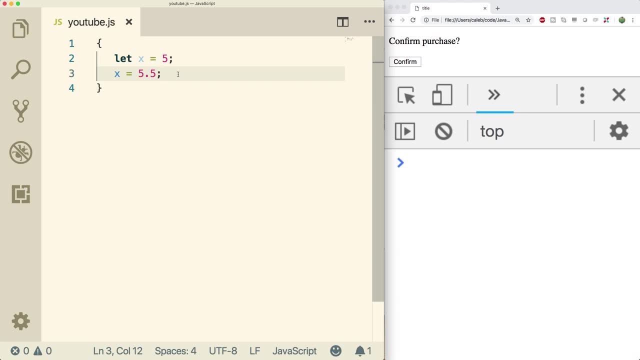 us a lot of memory to work with these numbers and allows us to do a lot of work. So if you store some pretty large numbers But there's only one data type for numbers- There's not one reserved for integers and there's not one for floats- and then double and then decimal, or 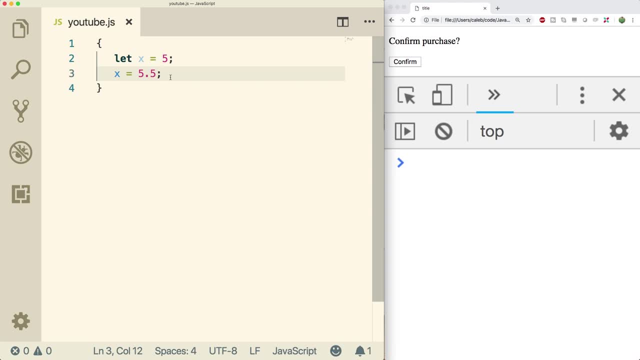 whatever it is, There's just number. Why is this important? Well, sometimes, when you're working with integer values, which basically are just numbers without anything with a decimal, it's important to make sure you are very precise and that the number you're trying to represent is. 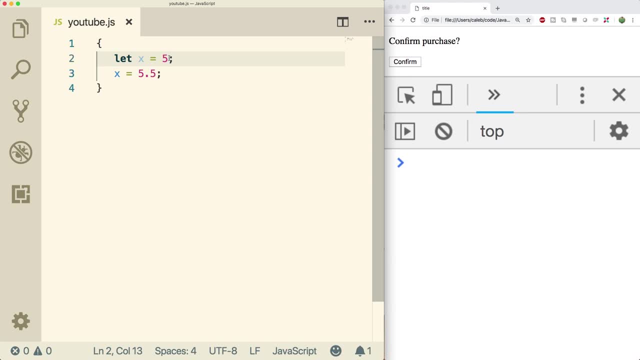 100% correct, But this is not always the case with a floating point number. Because of the way JavaScript stores numbers, you can occasionally get some odd things going on with your numbers, And this is going to happen when we try to go too high in our number or too low. So if you 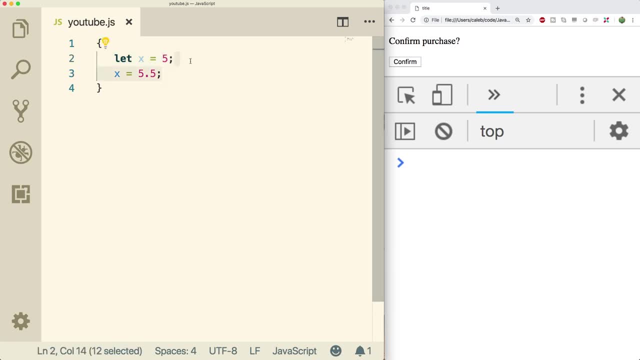 wanted to safely store an integer. how high could you go? Well, you can actually figure that out using number dot. and then there's this max safe integer and min safe integer. So let's print the max safe integer for a sec. We do a refresh and we get this huge value. Let me zoom out. 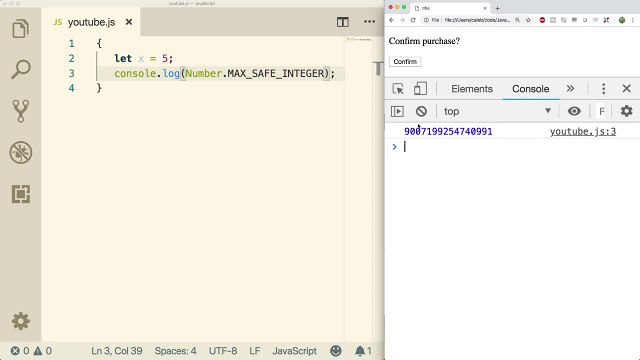 That's the value. So if you're storing dollars to represent your bank account, congratulations, but this is the highest integer we can safely store. So what exactly do I mean by safely? Well, check this out. If we do something like we console log x, we should get that value And 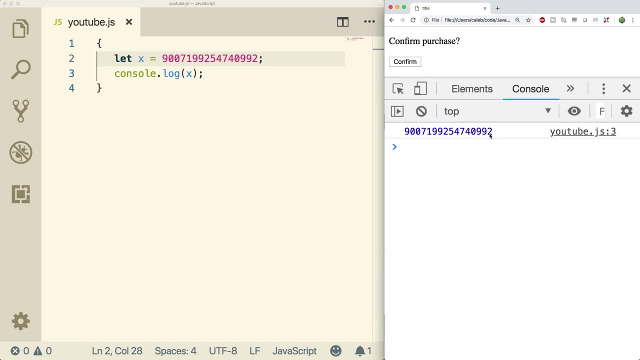 now. let's increase it one, Print it, we get two. Let's increase it one more. Do refresh. Oh what? Huh, We're still getting two, even though we put the value three. Oh, that's weird, We put four Now. 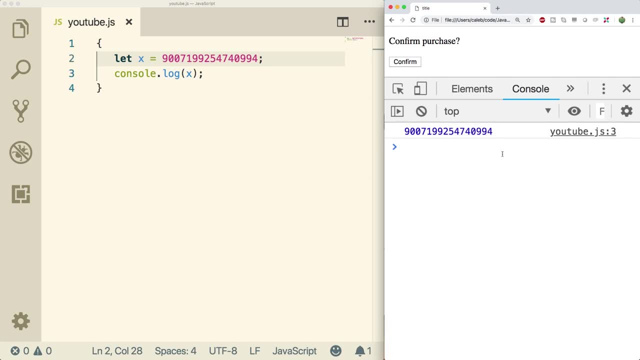 we get four, Okay, so we can't put a three there? Exactly That's what I'm trying to say. Not all numbers can be represented once we get into the large numbers. That's because we're given a limited number. That's because we're given. that's because we're given limited space and memory to store our 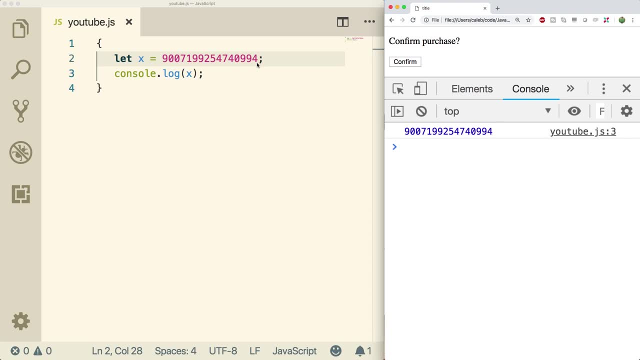 number, So we can't just create infinitely large numbers. we can test if a number is in the safe zone. Using number Is safe integer and putting the thing we're testing inside of parentheses. do a refresh. we get false. So anytime we get false for this, we know we're in the issue zone If we bring this. 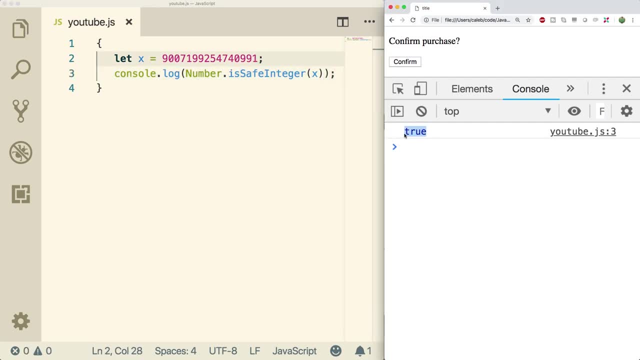 down to 91, we should be okay. And there we go. Now you can store really large numbers and you store really small numbers, But sometimes you might want to just represent infinity, And you actually can do that with number because there's three special values with a 64 bit number, That's. 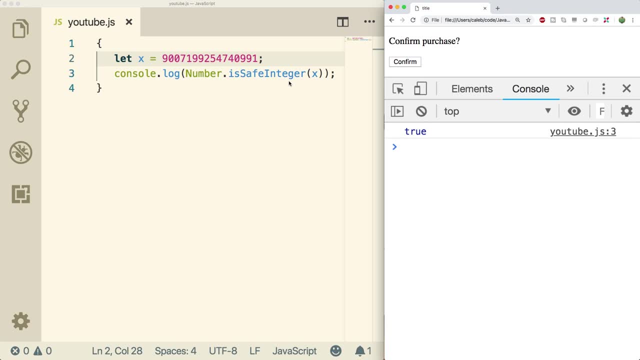 really cool Instead of zero, provided we put the function in And then a maximum or constant value like zero, So it's the same thing. So we can't do this. There's no negative infinity. there is infinity, negative infinity and not a number. So yeah, not a number as a possibility for the number data type. 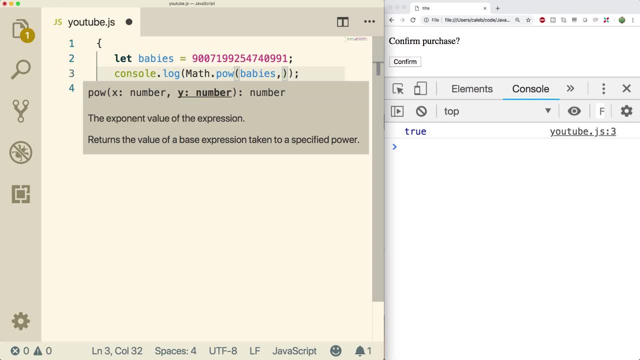 So, for example, we're just going to go through a little application raised to a power, then we put a comma and then the exponent. So you know, I want lots of babies. so we'll raise it to the 200th power And what's going to happen is, when we refresh, we just get. 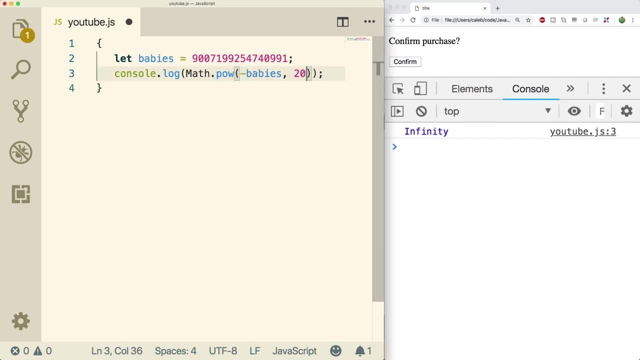 the value infinity. Same thing. if I want a negative number, that's possible if you get these inputs correct. Boom, negative infinity. This works like normal infinity. For example, we can multiply it by two and it's still infinity. Now the other special value is not a number And this will 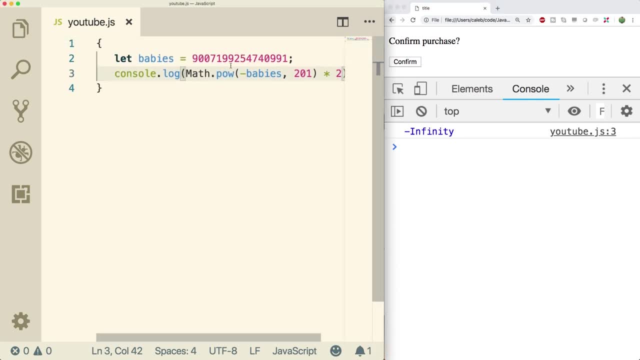 occur if we're trying to do math on something that doesn't really make sense. So, for example, let's try to add two to console dot log. So we're printing console dot log plus two. When we do a refresh we get not a number, which makes sense, because how are we supposed to add two to console?